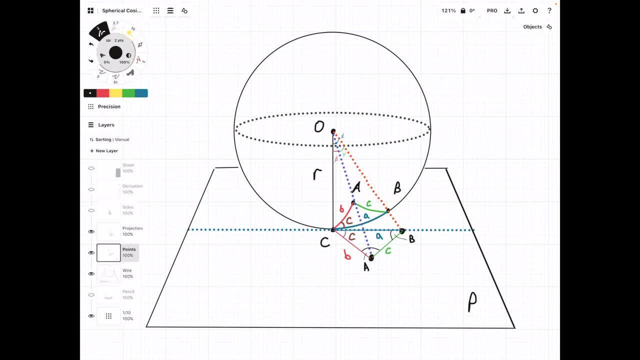 But we can see that when we do this, we have a projection line like this and a projection line like this. Each of these arcs say arc B. They are technically on a great circle. So if I draw this out freehand here, a great circle could look something like this: 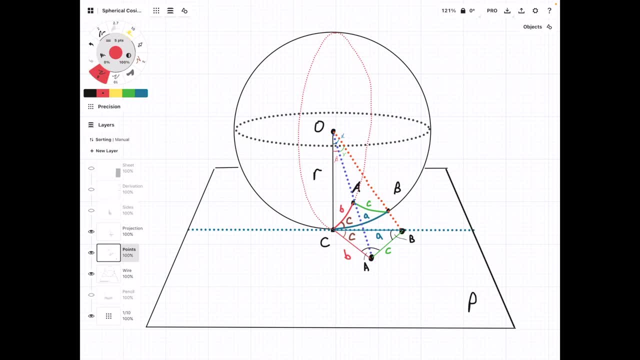 And a great circle is simply the intersection of a plane with a sphere that passes through the center point. And I say plane because it's not just contained in the sphere, it's in this giant plane that's outside of it. And when you project a plane, it has a center point. 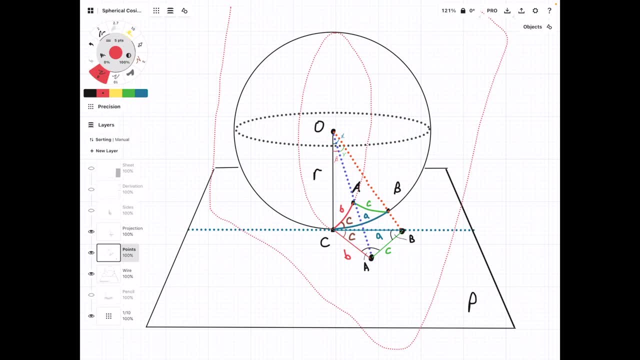 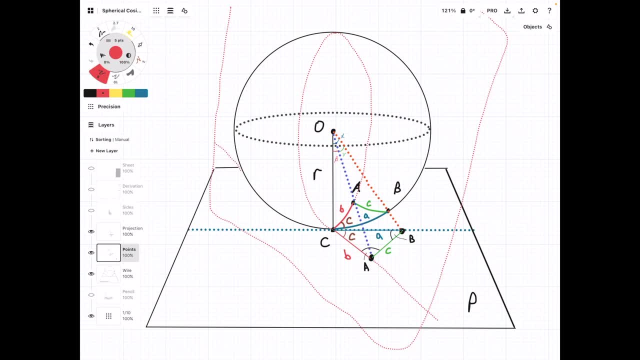 actually gonna form a straight line like this, so there's gonna be this line carrying all the way through. I can do the same thing for arc C like this, so C's great circle could look something like this. and again, when we extend it out through this plane, we have a plane like this and it's kind of formed this. 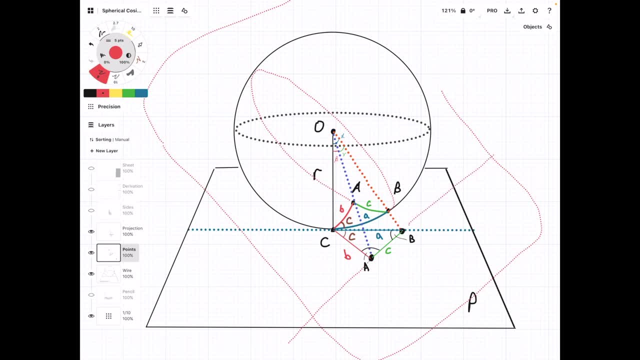 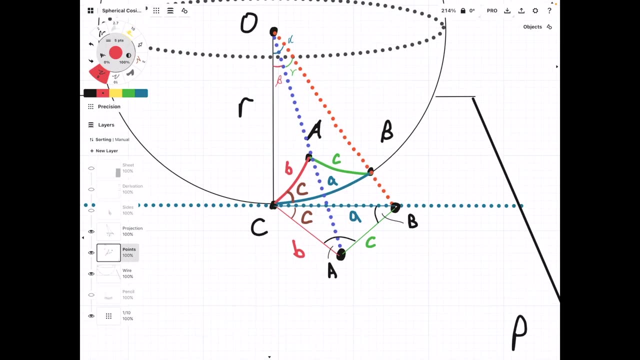 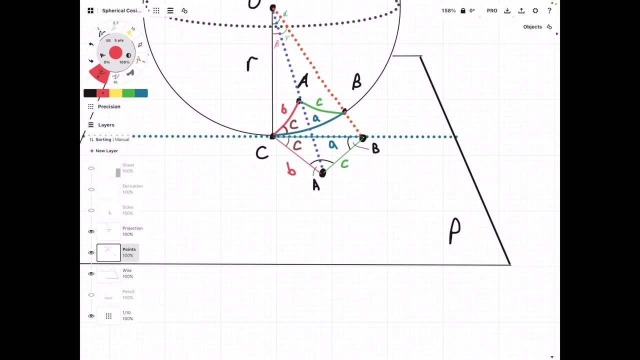 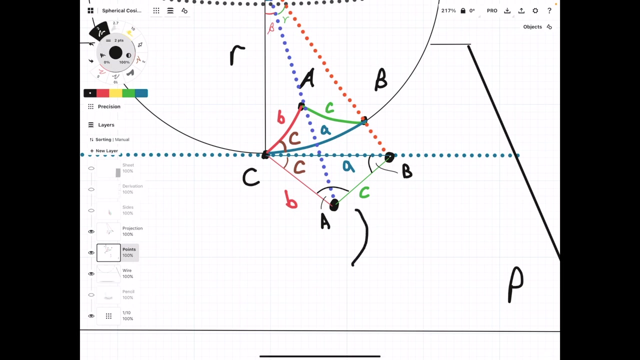 circle this line here where it intersects, where the planes intersect. okay, the point of all that is to say that when these great circle planes intersect, this plane P here, we're gonna have a regular planar triangle from so this triangle here. so The sides are not arced, they're straight lines and we can deal with it using the trigonometry that we already know. 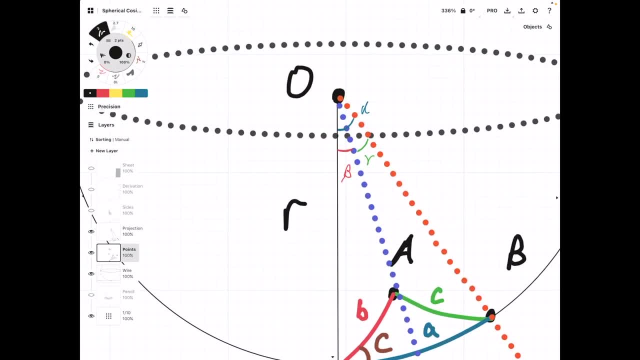 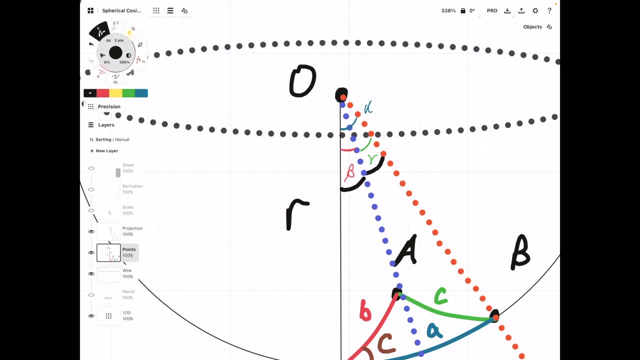 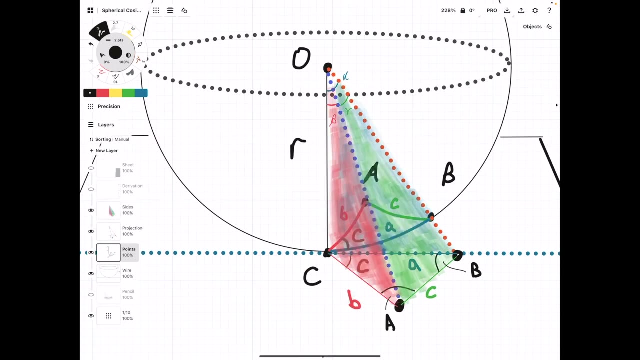 One other thing to point out about this is that we have a few angles here extending from the center, So we have angle beta, which is here, angle gamma, which is in the front, and then angle alpha in the very back. I've added a little bit of shading like this to show you the sides of this pyramid that we're kind of forming. 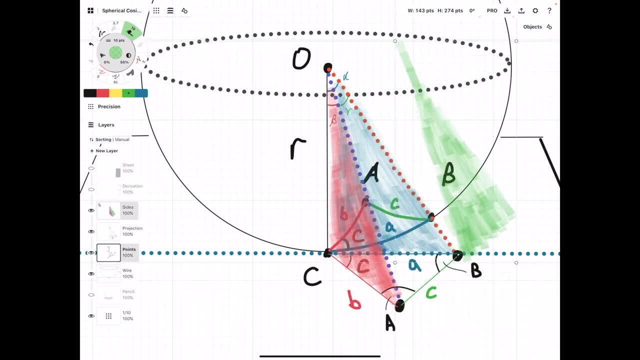 So I can pull off the front. this is like the front side of the pyramid, and then we have the side here And then the back. that blue triangle is on this blue line, so it's in the same plane as that. Let's put the sides back on. 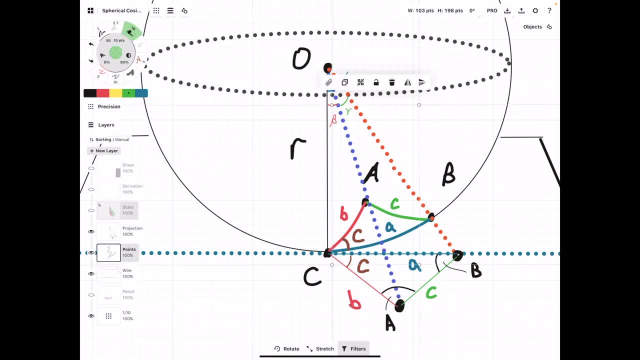 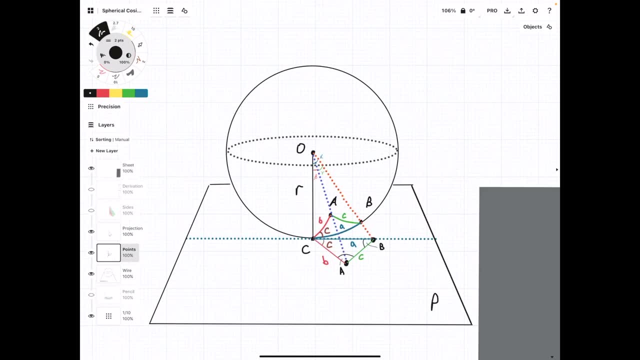 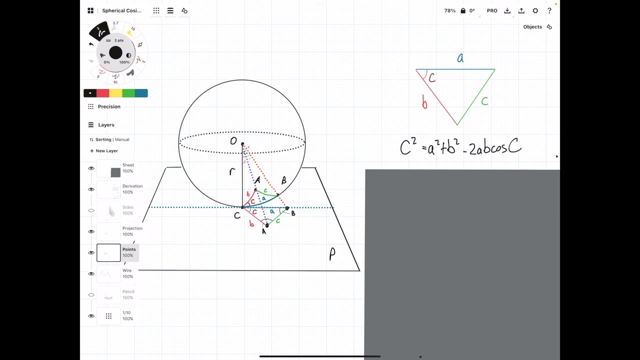 Alright, and I'm going to hide this because it kind of gets in the way, Oops. So now we're going to jump into the derivation. I have a little big rectangle here so I can block out all the different steps, But what we're going to do, the goal of this right now, is to find this length C. 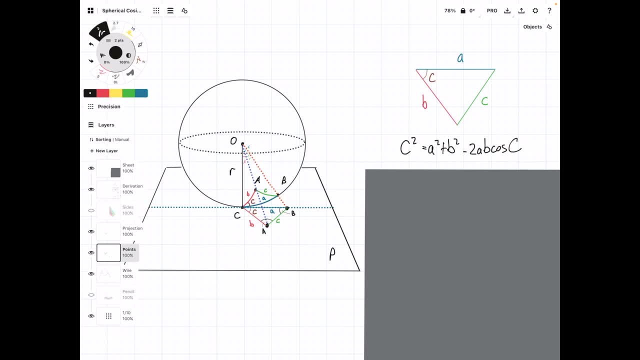 So when we Draw out the triangle that's on the plane, this is what it's going to look like. And again, it has straight lines. Oh no, It has straight lines for each of the sides and we have this angle C, that's across from side C. 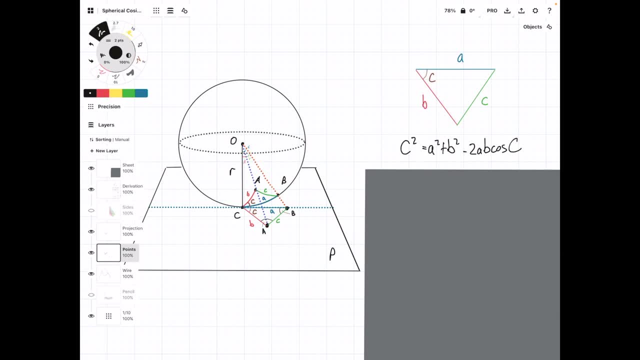 Because it's a regular triangle. we can use the regular, regular law of cosines, which is: C squared equals A squared plus B, squared minus 2AB cosine C. The problem is we don't know what A or Or B is. 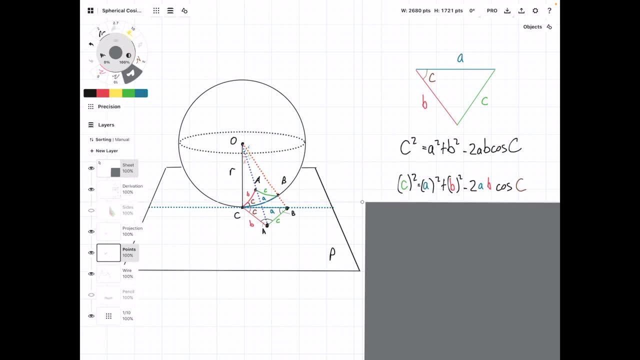 So we need to figure that out, And so, actually, this step: I just show how we're plugging in the values that we have, even though we don't know what they are, And then this step is how we figure out what they are. 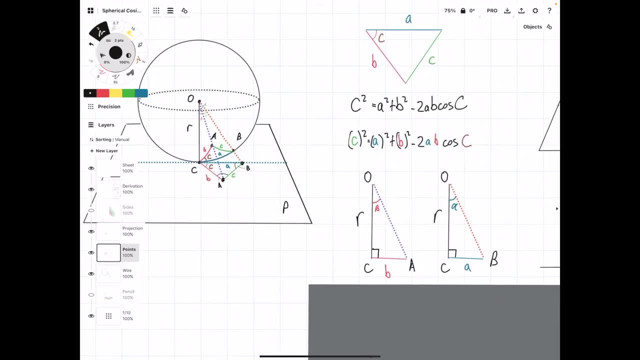 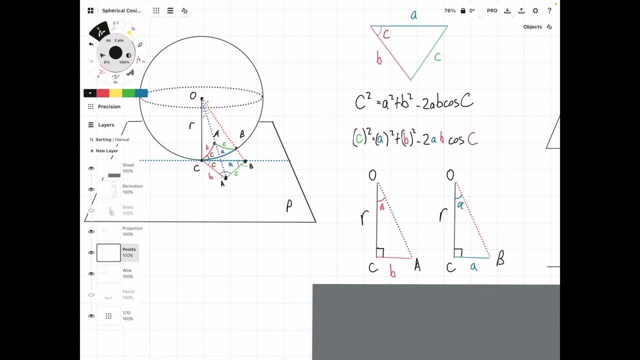 So, in order to figure out what sides A and B are, we can use the fact that this triangle here that I'm shading in is a right triangle, And so is the one in the back that is made by OCB, And so I've basically taken these two triangles out of that diagram and I've put them here. 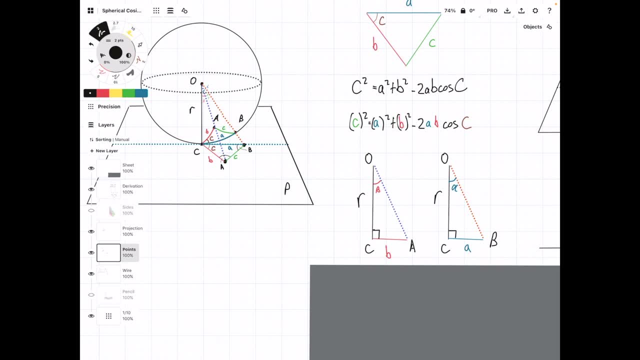 So this is what they look like if we're looking at them from the side. We have a right triangle at the very bottom where the two planes, or where the sphere and its tangent plane come in contact, And then we have the angle alpha. 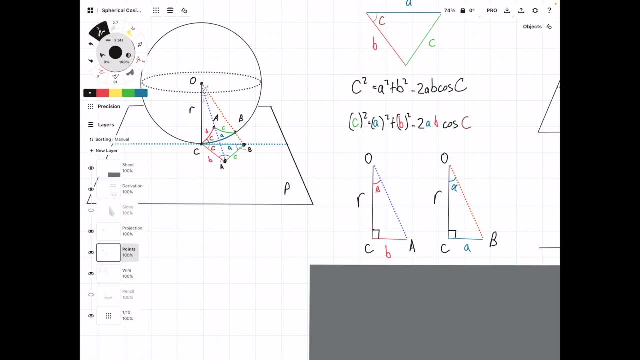 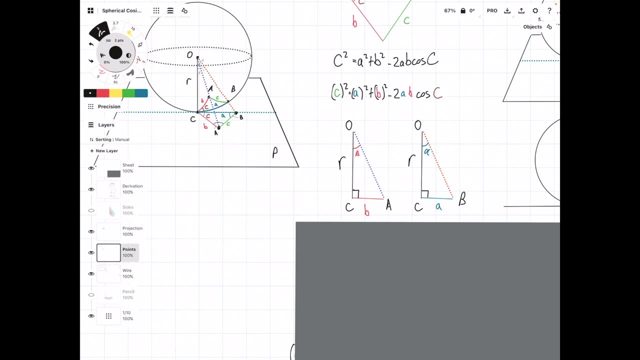 And the angle beta up top. And then what we're going to do is we're going to treat each of these triangles separately. Well, not separately, We're going to do the same thing to each of them. We're going to use the Pythagorean theorem to figure out what side B is. 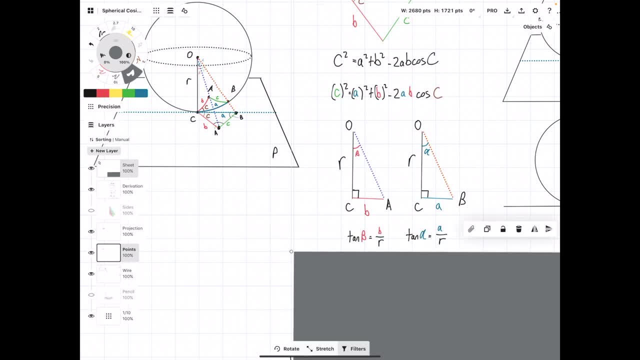 So, because we know the side is the side R, we have B on the bottom, We can do: tangent of beta equals B over R and tangent of alpha equals A over R. We'll solve for B and A like this, And then, as I mentioned, this is a unit sphere, so R is equal to 1.. 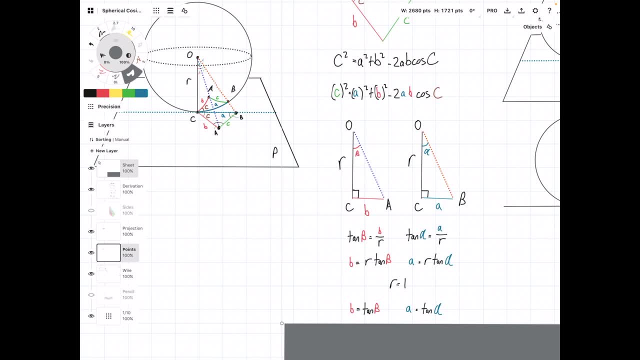 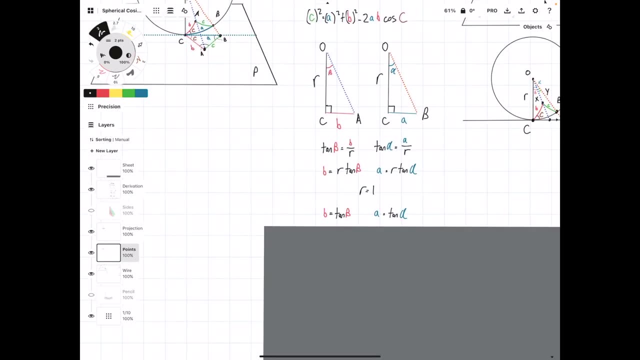 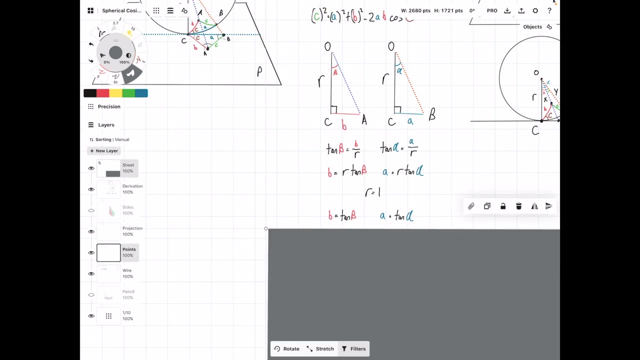 So we can simplify this to: B equals tan beta and A equals tan alpha. So we're doing pretty good here. Now what we're going to do is plug in these values into our law of cosines from before. So let me grab this thing and slide it down. 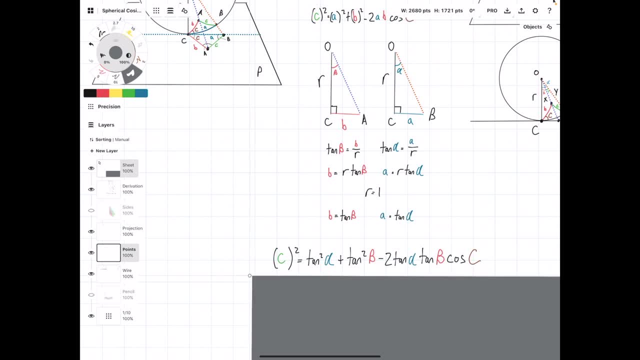 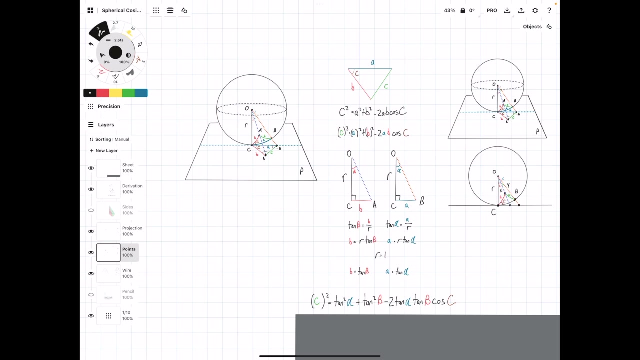 So now we have C squared equals tan squared alpha, plus tan squared beta, minus 2 tan alpha, tan beta cosine of C, And so what I did here was went back up to this triangle And now we're solving for side C: Move that pin. 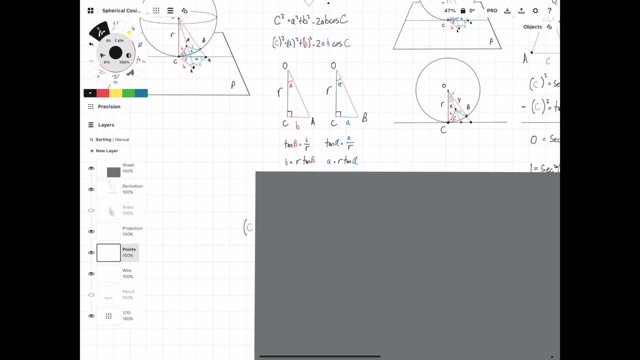 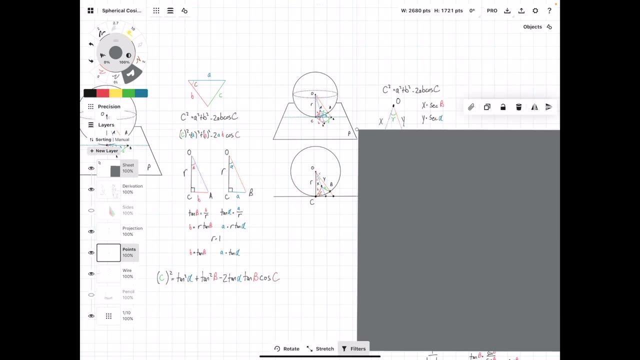 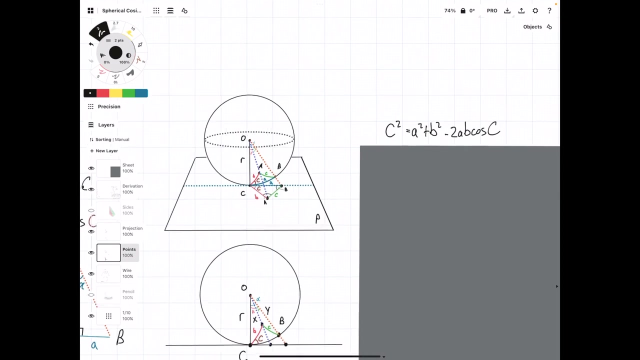 All right, that's the last step of that one, So now? So now, next step: zoom out here, bring this over. Sorry, this is a little clunky, but it helps with explaining. All right, so now what we're going to do is we are going to look at a different triangle. 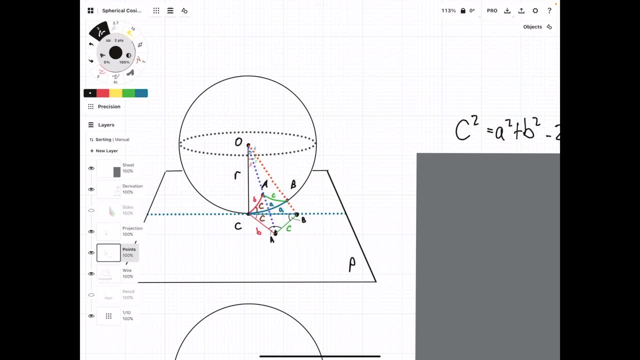 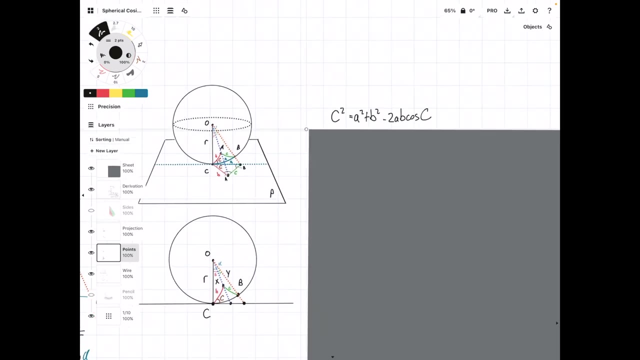 that shares this side C And that triangle is going to be the one on the front face right here that I'm shading in. So the two lines that get projected down they form another triangle. So again, we're going to use our law of cosines to figure out what side C is. 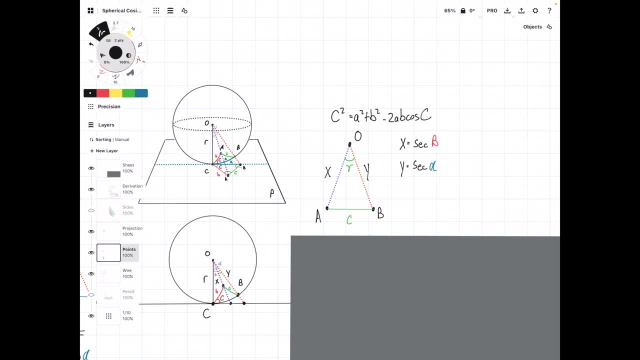 And so here, just to help you visualize, I drew out this triangle on the front Again, for the sake of being clear. it's this triangle here, And the interesting thing, and a very useful thing, is that the line that extends from the center of the sphere 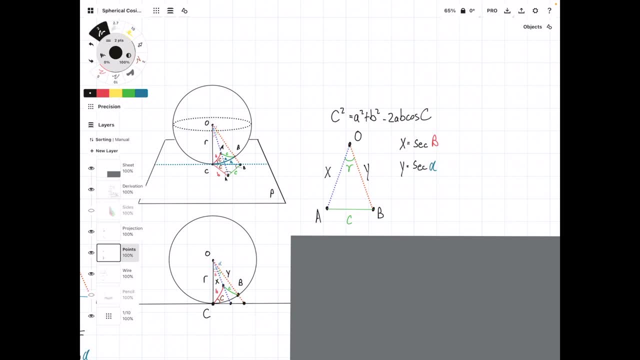 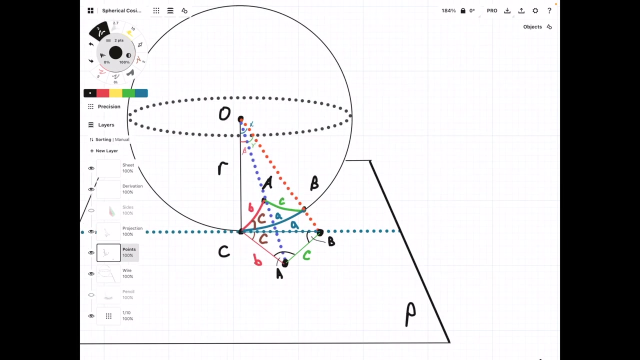 and intersects with the tangent plane. so this line and this line, those are both secant lines And they're defined by the angle that they're formed by. So you have alpha in the back and beta in the front. I can put a helpful 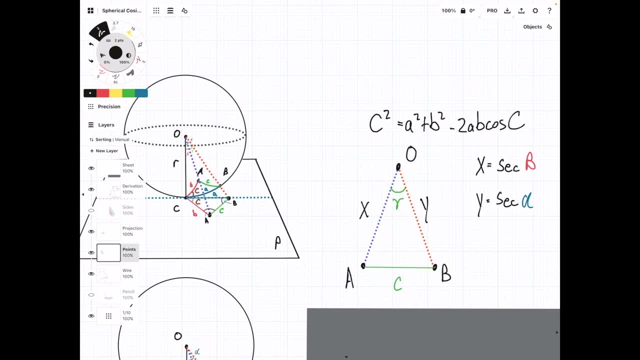 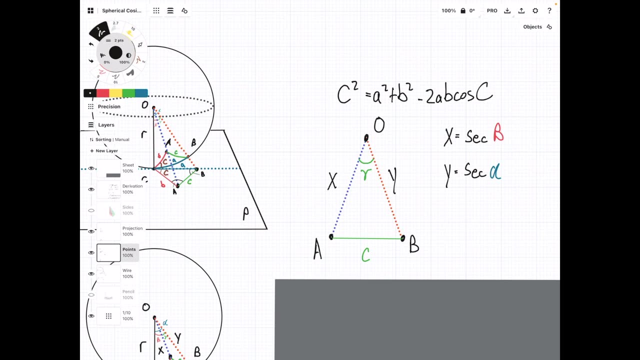 I can put a helpful link in the description of this video to help you see what a secant line is. But for the sake of this derivation, we know that x is equal to secant beta and y is equal to secant alpha. 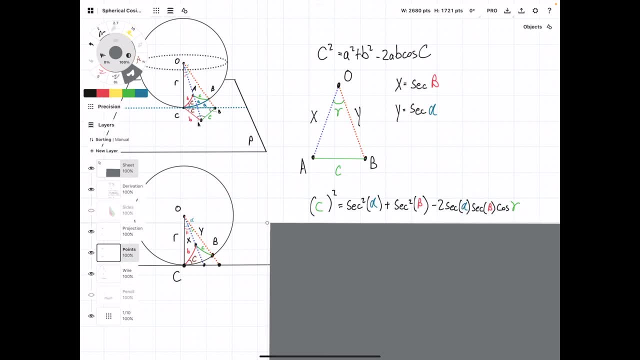 Okay, Now we can sub in the values that we need into our law of cosines. So c squared equals secant squared alpha plus secant squared beta minus 2 secant alpha, secant beta cosine of gamma. And so we are using everything that we're given. 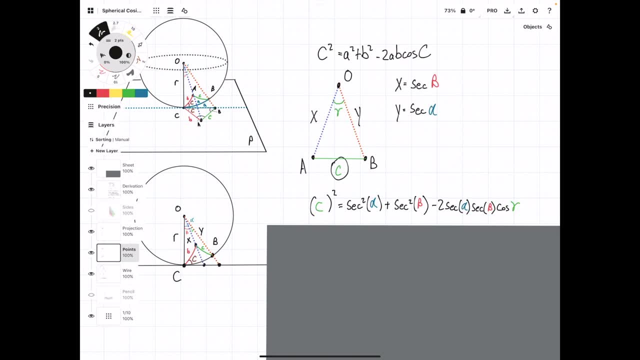 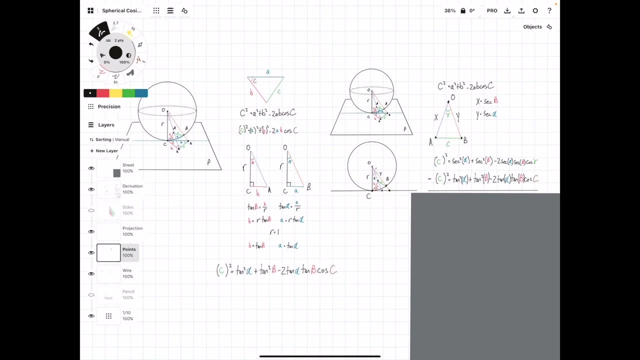 in this triangle to solve for this law of cosines. We have side c across from angle gamma, So we're using that. Then, what we're going to do is we're going to take the formula from the first part, this one where we also solve for c, squared or c. 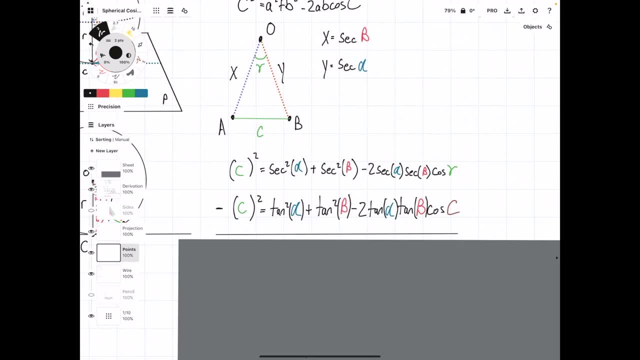 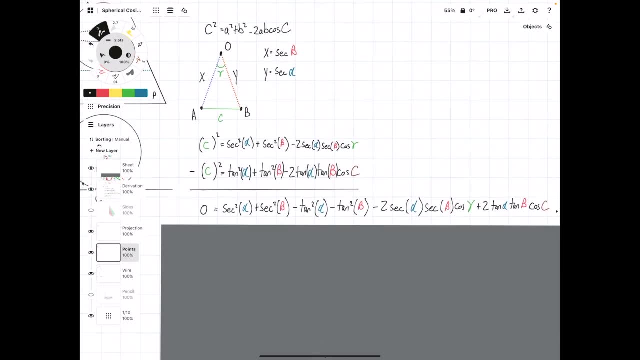 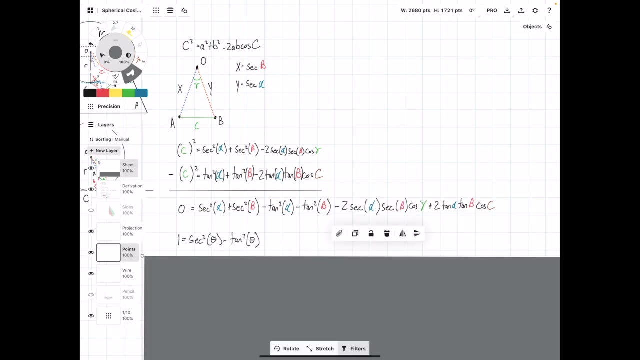 and we're going to subtract it from the equation we just found. So when we do that, we get this giant statement here. I'm not going to read it all out because it's a lot, but we can use a trig identity. 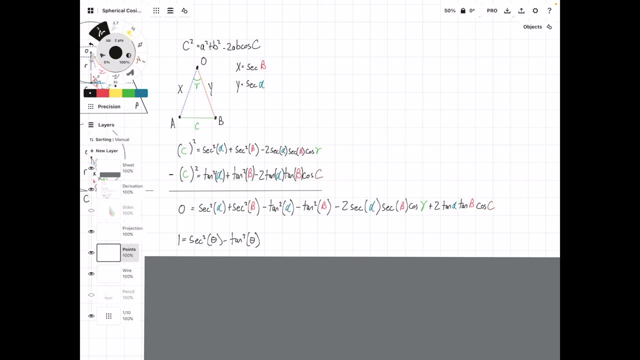 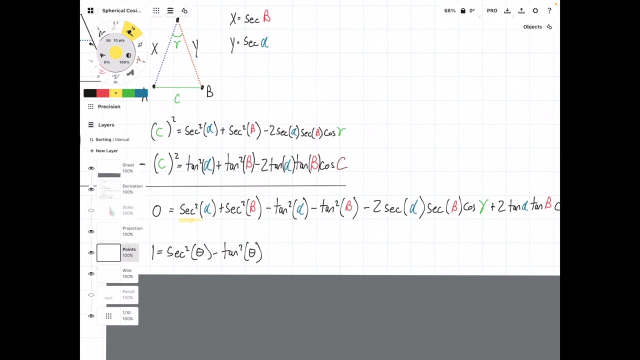 which is 1, equals secant squared beta minus tan squared beta, to simplify this. So here what we have is we have two pairs of secant squared minus tan squared. First one is secant squared minus tan squared, alpha, And then we have secant squared. 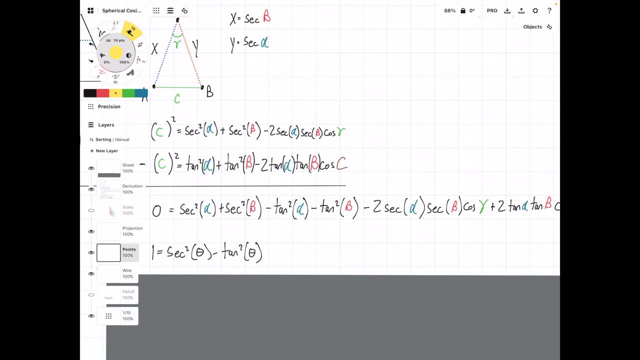 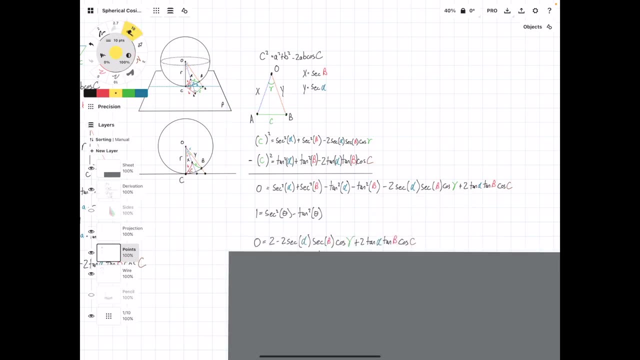 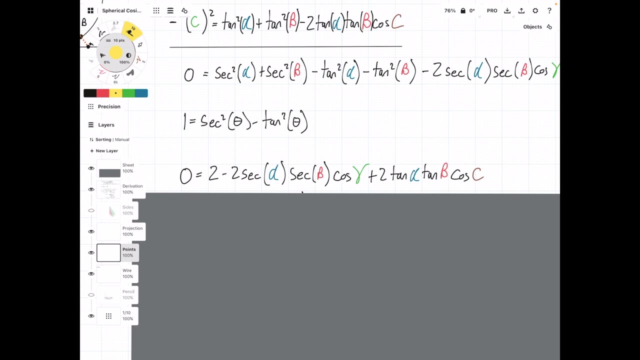 minus tan squared beta, And so both of those just turn into 1.. So the equation becomes this: Let's zoom in a little bit: 0 equals 2 minus 2 secant alpha, secant beta. cosine of gamma plus 2 tangent of alpha, tangent of beta. 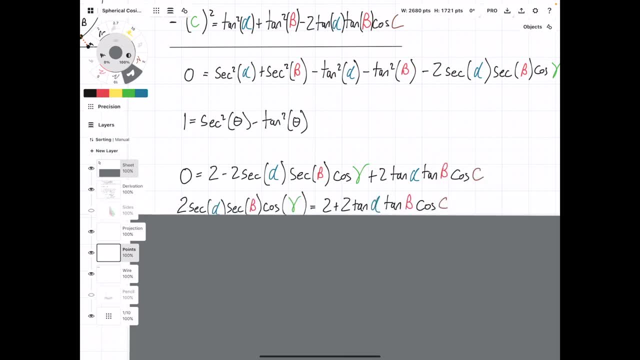 cosine of c. So we're getting somewhere. Now what we're going to do is we're going to try to solve for cosine of gamma. So what I did here was just bring. Oops, Okay, Not cooperating with me. So all I did here was I took. 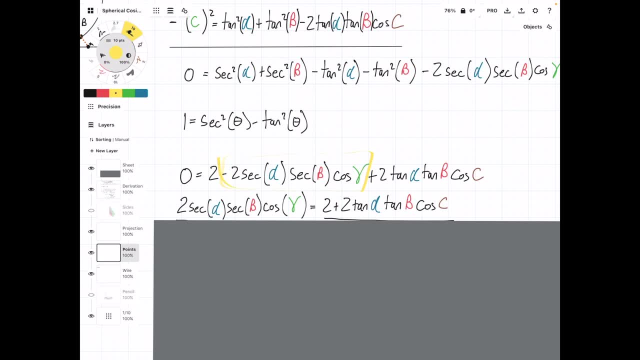 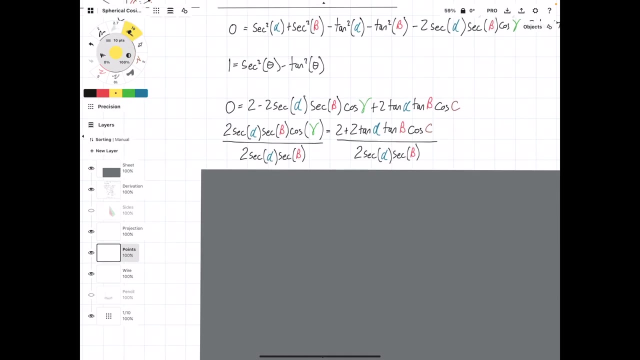 this portion of the equation and I took this one formula and I brought it to the other side, And then I'm going to divide by 2 secant alpha, secant beta to get cosine gamma alone. Keep going down, And then this is what we're left with. 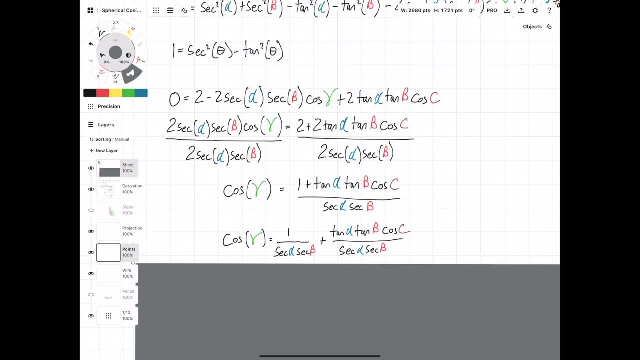 And then we can separate it into. we can separate the right side into two different elements. So 1 over secant alpha secant beta plus tangent of alpha, tangent of beta. cosine c over secant alpha secant beta. 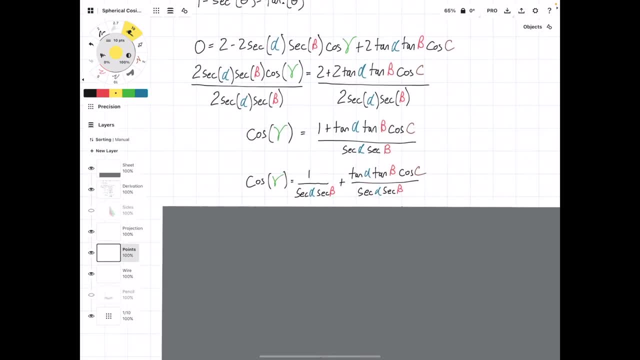 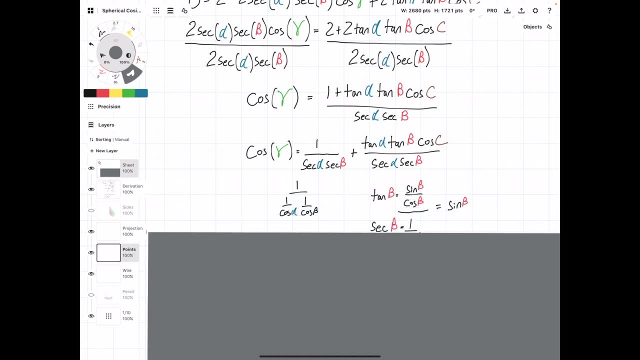 All right. Next step is to turn the right side into terms of just sine and cosine. So I do a little bit of like work here to show how it works, Work to show how it works. Yeah, So for the first element here. 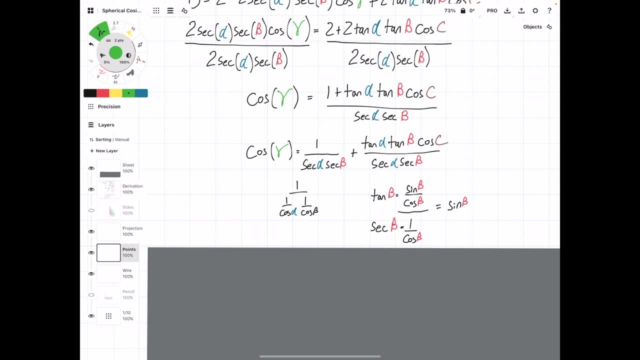 let me just grab a different pen. This whole equation or function here is equal to 1 over 1 over cosine of alpha, 1 over cosine of beta. So yeah, secant is 1 over cosine. And so let me just move down and actually it'll help to see what happens. 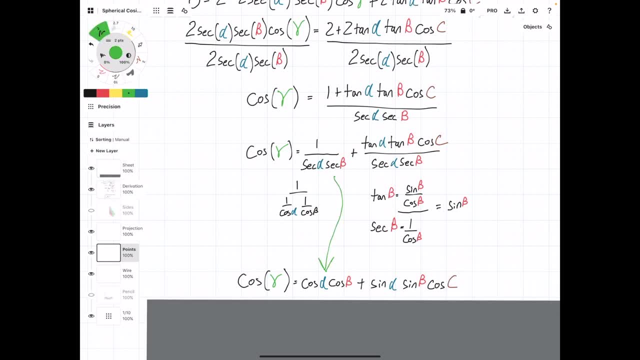 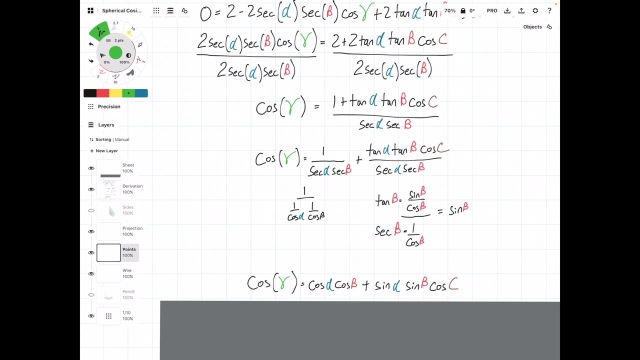 So the whole first element here turns into cosine, alpha, cosine beta, And then for the right side tangent of alpha over secant of alpha. that just becomes sine. And so I showed how that works here, And we have two pairs of this. 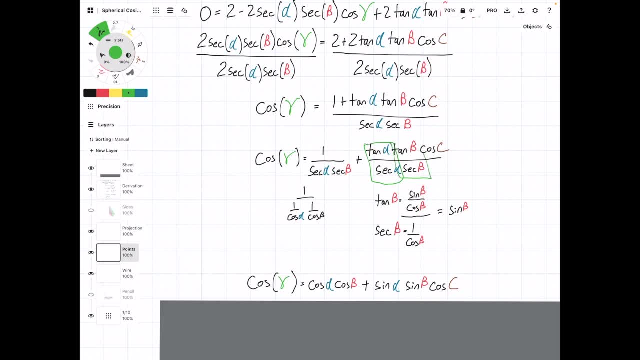 So we have the alpha pair and we have the beta pair, And so the right side just becomes this Sine of alpha times, sine of beta, beta. And then we have cosine c, And so we're not quite done, As I've mentioned several times.